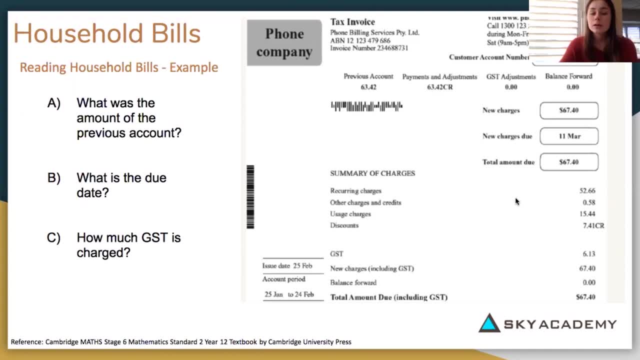 So you pretty much need to know just how to read this bill. So we'll go through and have a look at reading it now by answering these questions. So question A says: what was the account, What was the amount of the previous account? So to answer this question, you just look at the bill and you 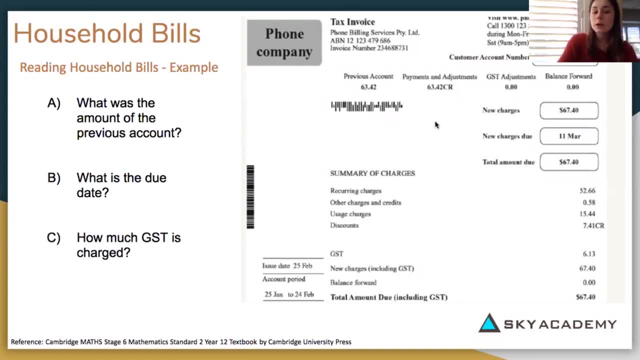 have to find the section where it says previous account. And so if we look up here here, it says previous account and it has a money associated to it, It has a value associated to it, It has a value associated to it, And so the value or the amount of the previous account was simply $63 and 42 cents. 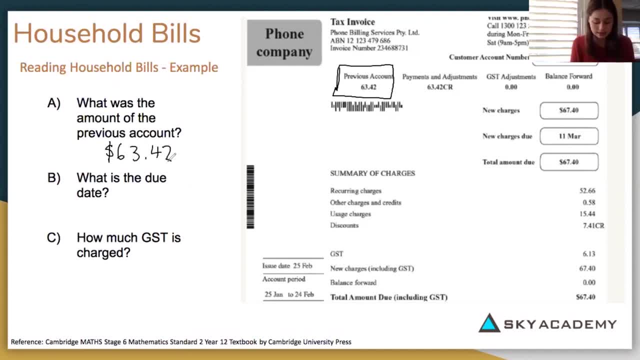 So, as you can see, there's not really any working out associated to household bills. It's just reading the bill and understanding what each thing means. So if they want the previous account, that just means that the previous bill had $63. And so the only time you will have to do working out, for example, if they leave the GST app and you 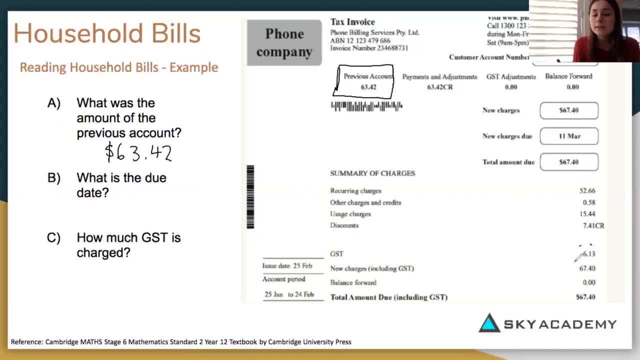 just have to calculate 10%, So they might have that here and they'll say: what is the GST? And then you'll have to look at the charges and then you'll have to know that GST is 10%, And then you'll have 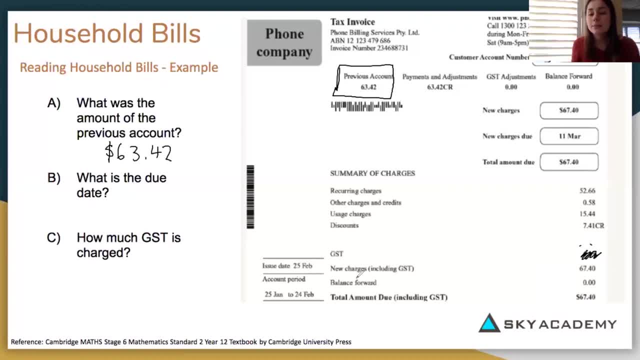 to calculate 10% to find the GST. Things like that might be a little bit more complicated. So if you're left off the household bill and asked you to calculate it, other than that it's just reading off the bill. So let's have a look at question B. It says what is the due date. So if we have a look, 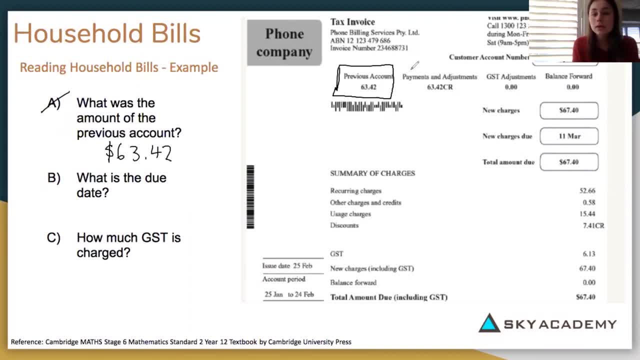 and do a quick scan all across the bill we come to here and the new charges, not the ones we did previously, not this account here, But the new charges are due on the 11th of March, So the due date is simply the 11th of March.